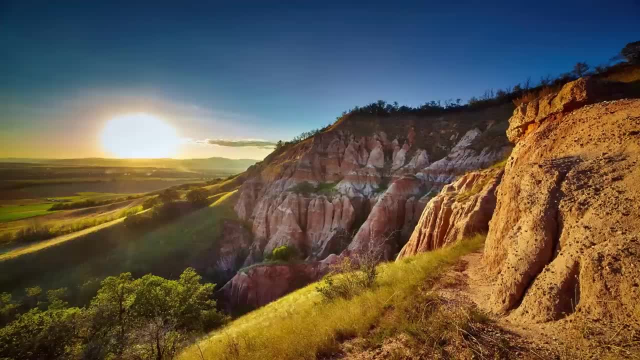 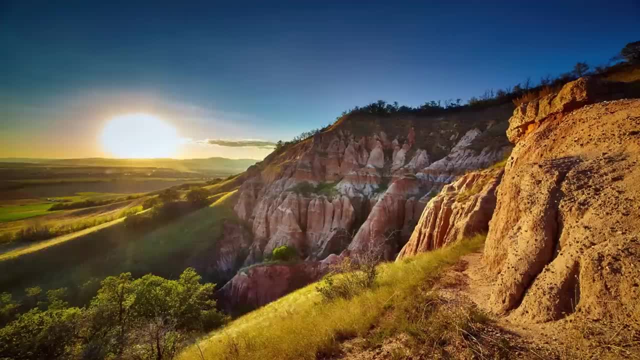 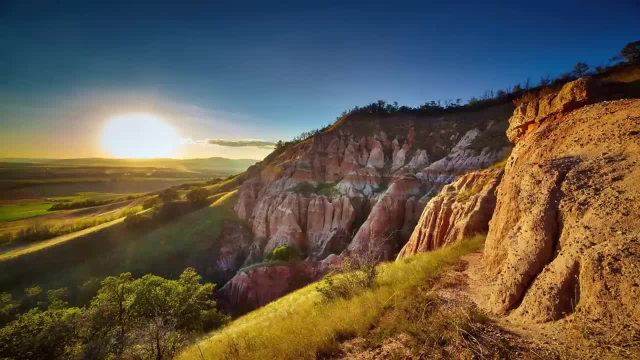 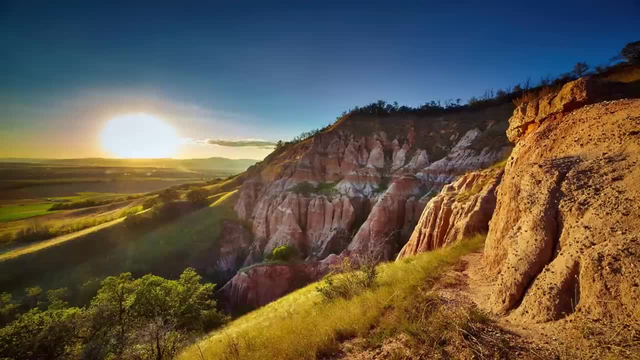 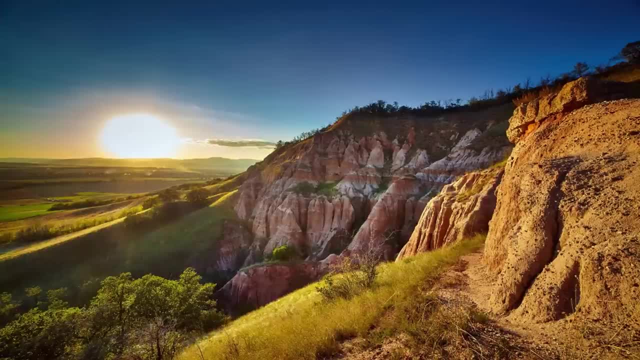 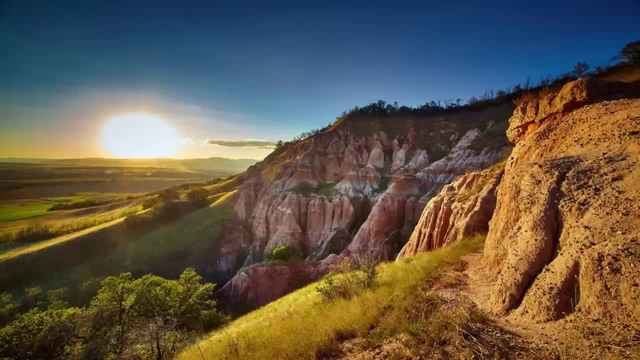 and release tension. With each breath, I relax my muscles in my body and release tension. With each breath, I relax my muscles in my body and release tension. I am filled with the love of universal power within. I am filled with the love of universal power within. 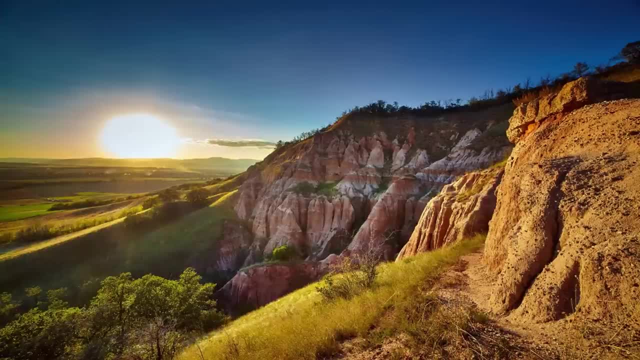 Today, I choose to release all barriers that are holding me back. Today, I choose to release all barriers. I choose to release all barriers that are holding me back. My mind is now free. My mind is now free. I release any worries of unimportant things. 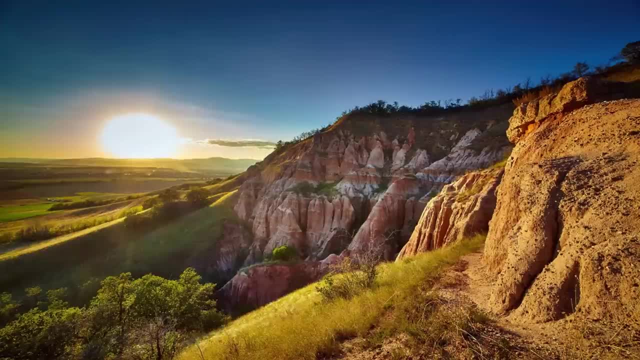 I release any worries of unimportant things. With every breath I take, I allow my mind to relax deeply. With every breath I take, I allow my mind to relax deeply. With every breath I take, I allow my mind to relax deeply. 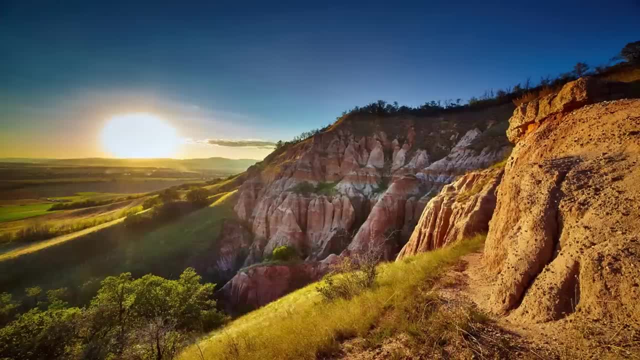 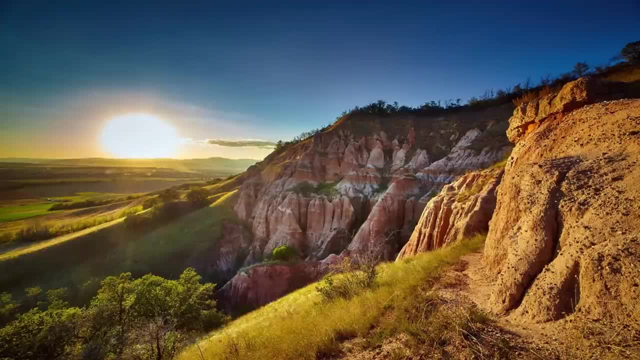 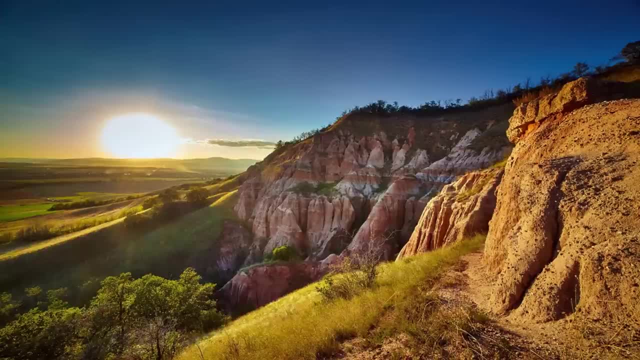 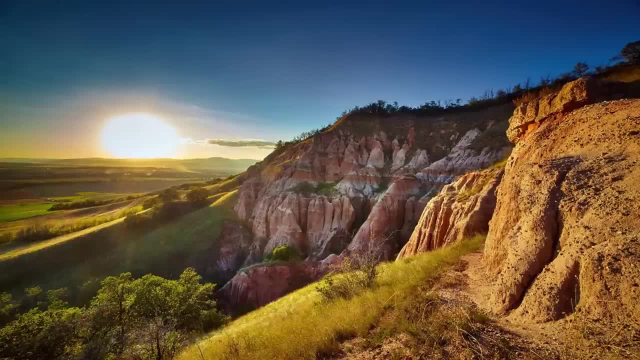 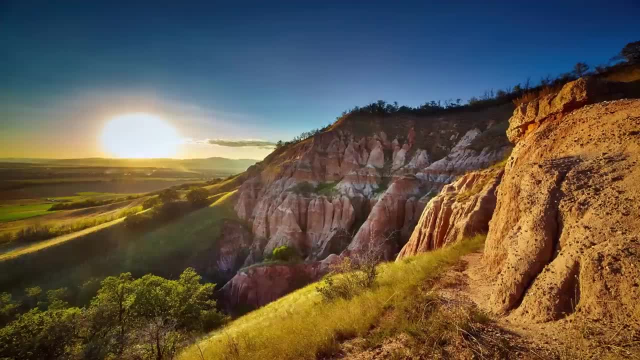 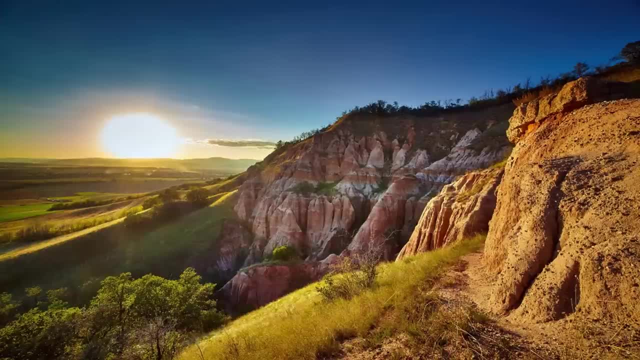 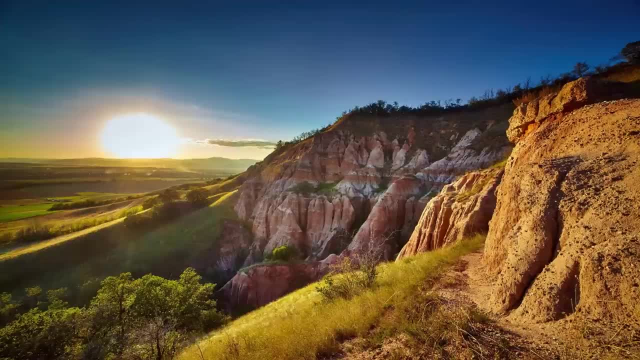 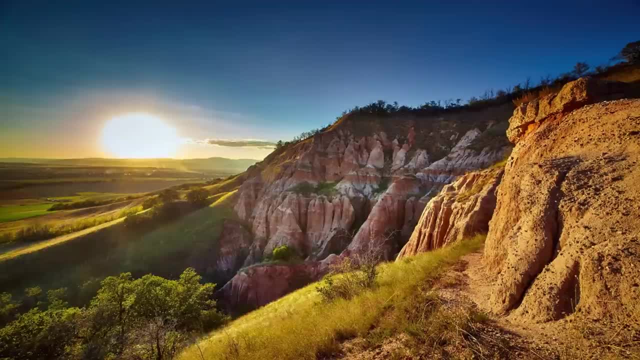 Each day, I awaken with an attitude of gratitude. I let go of all tension that is within me. I let go of all tension that is within me. I am open to a deep calmness inside me. I am open to a deep calmness inside me. 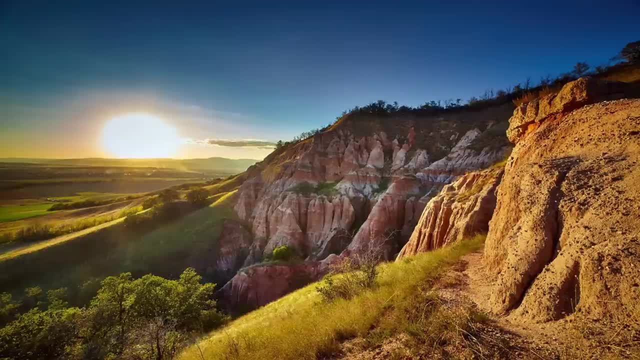 Right now, I relax my shoulders. Right now, I relax my shoulders. Right now, I choose to be at peace with myself. Right now, I choose to be at peace with myself. Right now, I relax my shoulders. Right now, I relax my shoulders. 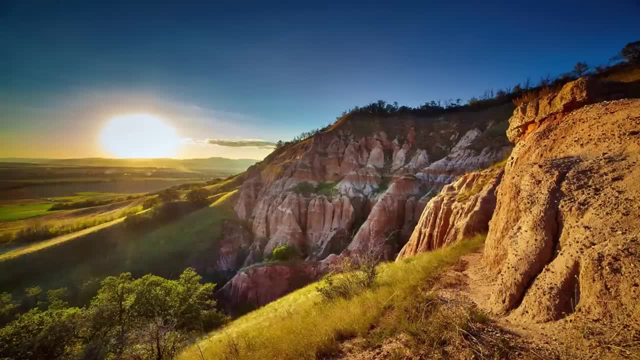 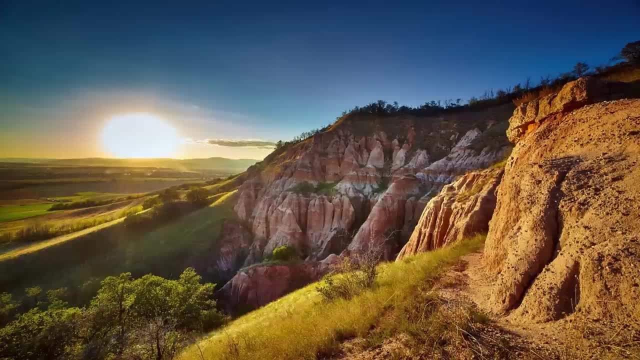 I allow my thoughts to drift to a positive and peaceful place. I allow my thoughts to drift to a positive and peaceful place. I'm making every effort to forgive myself. I'm making every effort to forgive myself and others. I'm making every effort to forgive myself and others. 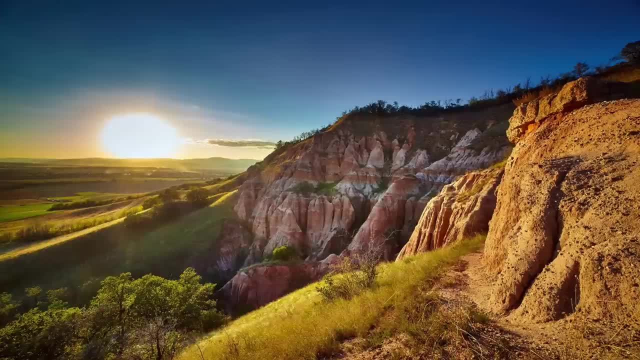 I am always in harmony with the universe. I am always in harmony with the universe. with each breath, I relax my muscles in my body and release tension. with each breath, I relax my muscles in my body and release tension, I am filled with the love of universal power. within. I am filled with the love. 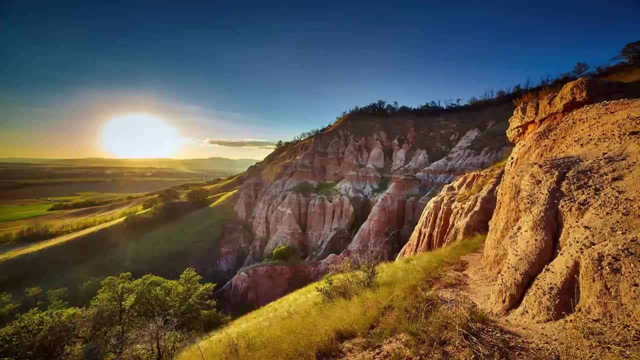 of universal power. within today, I choose to release all barriers that are holding me back. today, I choose to release all barriers that are holding me back. my mind is now free. my mind is now free. I release any worries of. I release any worries of. I release any worries of unimportant things. 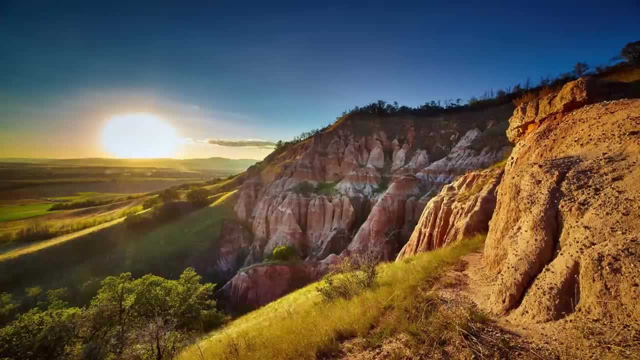 unimportant things, unimportant things. I release any worries of unimportant. I release any worries of unimportant. I release any worries of unimportant things with every breath I take. I allow my mind with every breath I take. I allow my mind with every breath I take. I allow my mind to relax deeply with every breath I. 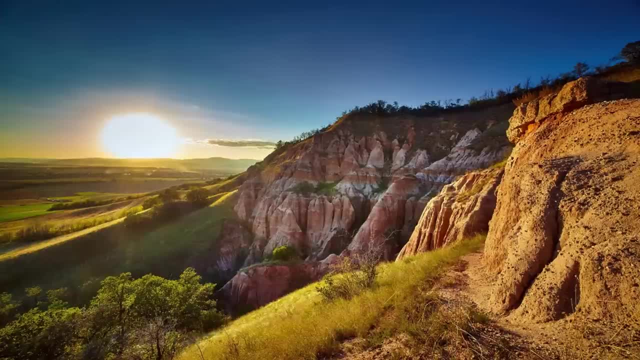 to relax deeply with every breath. I to relax deeply with every breath I take. I allow my mind to relax deeply. take I allow my mind to relax deeply. I choose to react in a positive way in all situations. I choose to react in a positive way in all situations. 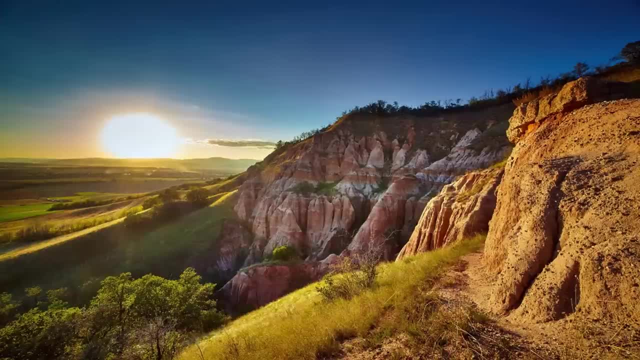 The things I don't like, I either accept them or can change them. The things I don't like, I either accept them or can change them. I am what I think, so I choose to think positive thoughts. I am what I think, so I choose to think positive thoughts. 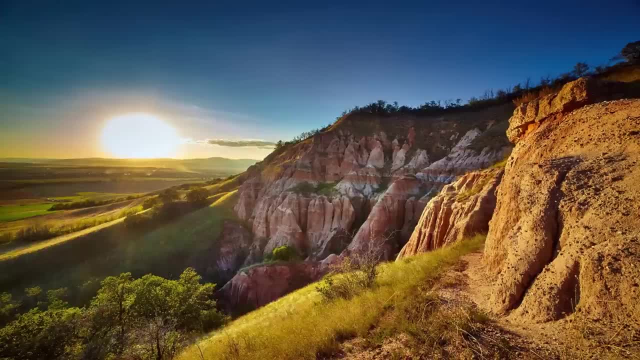 I am what I think, so I choose to think positive thoughts On each breath out. I release old negative thought patterns. On each breath out, I release old negative thought patterns. I am what I think, so I choose to think positive thoughts. 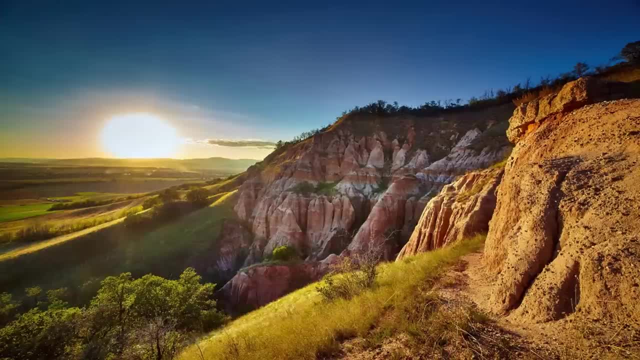 I am what I think, so I choose to think positive thoughts. On each breath out, I release old negative thought patterns. I am what I think, so I choose to think positive thoughts. I am what I think, so I choose to think positive thoughts. 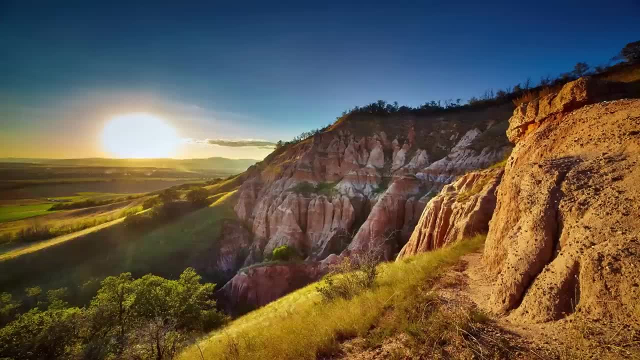 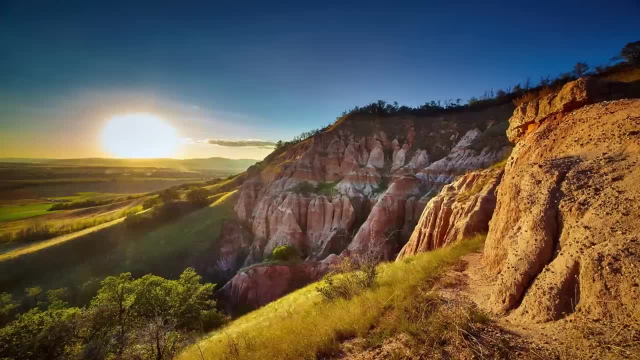 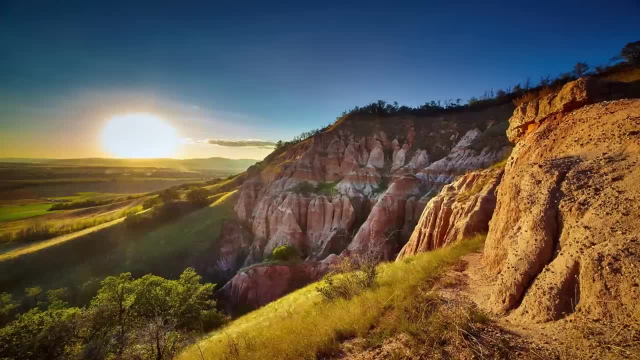 Things are going alright for me today. Things are going alright for me today. Tomorrow is going to be even better. Tomorrow is going to be even better. I create my own space for satisfaction. I create my own space for satisfaction. I choose to make happiness my number one goal. 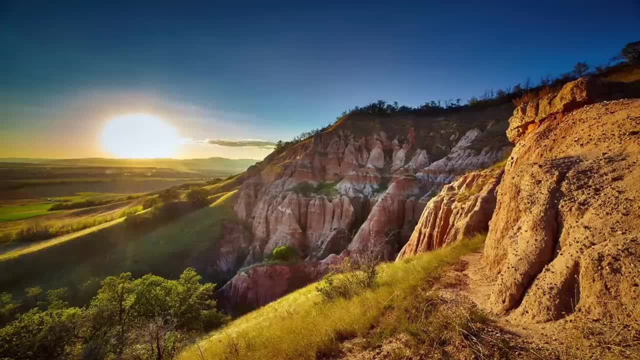 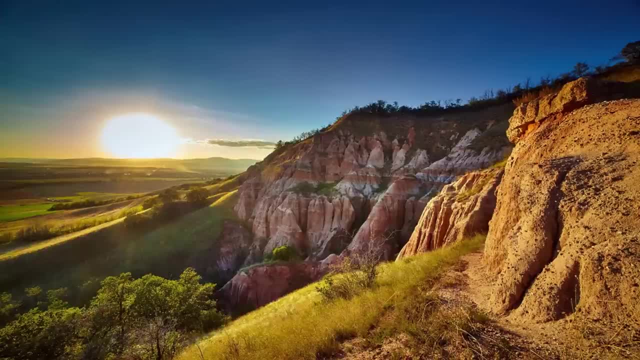 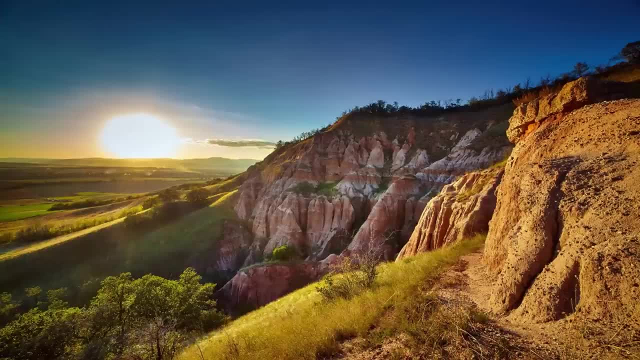 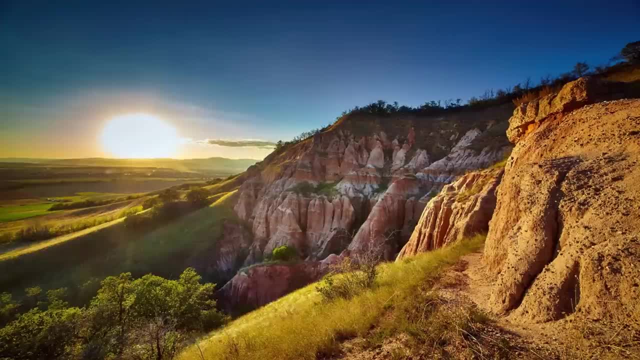 I am open to a deep calmness inside me. I am open to a deep calmness inside me Right now. I relax my shoulders. Right now, I relax my shoulders Right now, I choose to be at peace with myself. Right now, I choose to be at peace with myself. 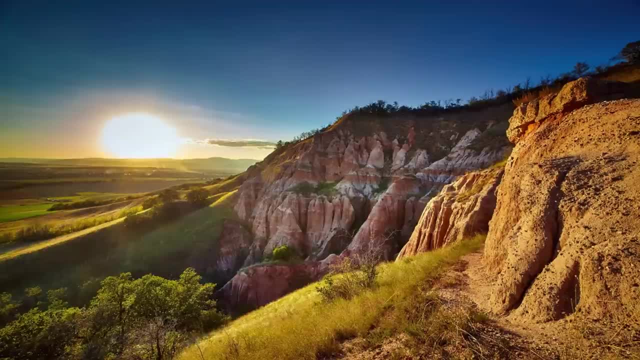 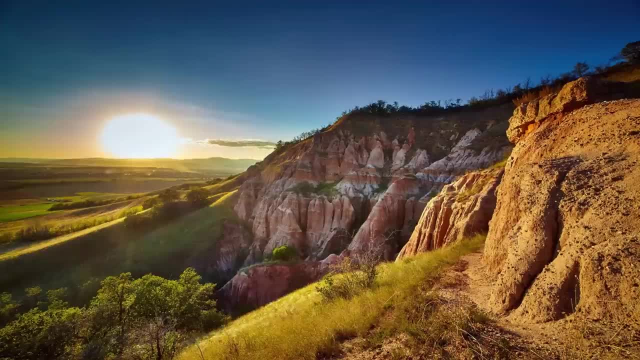 I release all thoughts that no longer serve me well. I create my own happiness in my life. I create my own happiness in my life. I allow my thoughts to drift to a positive and peaceful place. I allow my thoughts to drift to a positive and peaceful place. 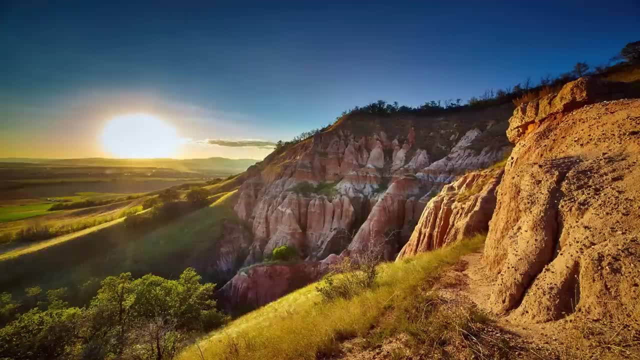 I'm making every effort to forgive myself and others. I'm making every effort to forgive myself and others. I am always in harmony with the universe. I am always in harmony with the universe. With each breath, I relax my muscles in my body and release tension. 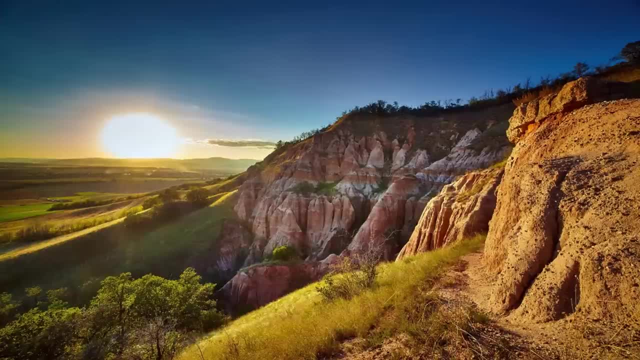 With each breath, I relax my muscles in my body and release tension. I am filled with the love of universal power within. I am filled with the love of universal power within. Today, I choose to release all barriers that are holding me back. 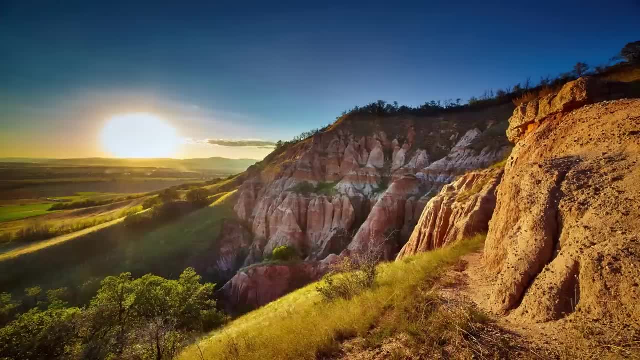 Today, I choose to release all barriers that are holding me back. My mind is now free. My mind is now free. I release any worries of unimportant things. I release any worries of unimportant things. I release any worries of unimportant things. With every breath I take, I allow my mind to relax deeply. 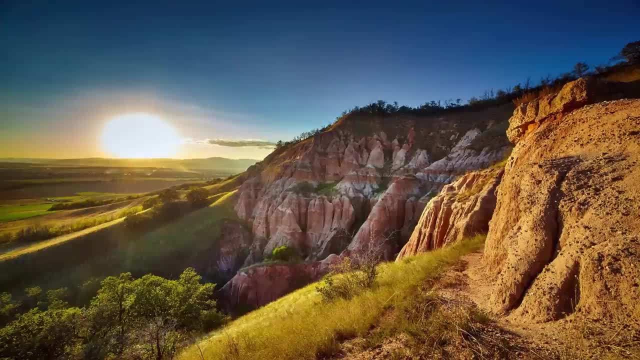 With every breath I take, I allow my mind to relax deeply. With every breath I take, I allow my mind to relax deeply. I choose to react in a positive way. I choose to react in a positive way, in a positive way in all situations. I choose to react in a positive way in all. 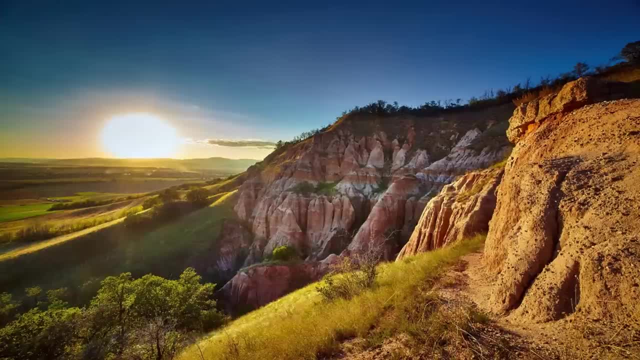 situations. the things I don't like, I either accept them or can change them. the things I don't like, I either accept them or can change them. I am what I think, so I choose to think positive thoughts. I am what I think, so I choose to think positive thoughts. 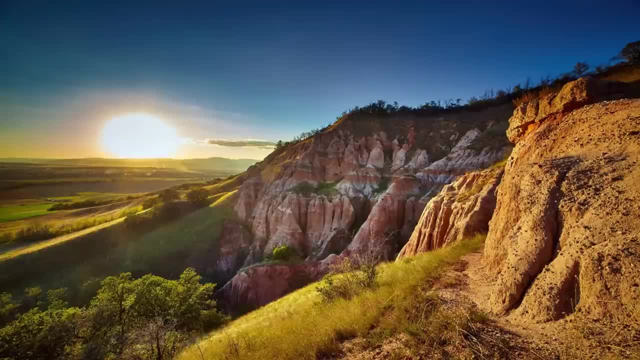 I am what I think, so I choose to think positive thoughts. on each breath out. I release old negative thought patterns on each breath. on each breath out, I release old negative thought patterns. I leave negative sentences, negativity behind. I leave negativity behind. Things are going alright for me today. Things are going alright for me today. 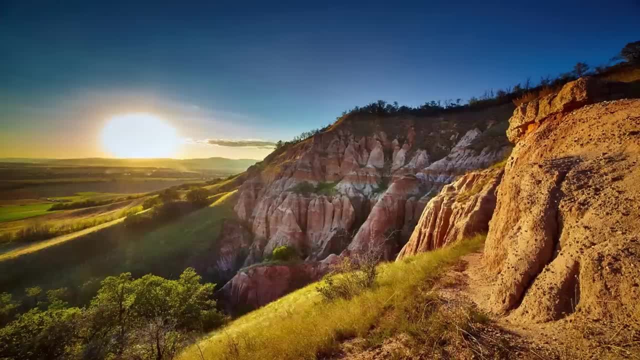 Tomorrow is going to be even better. Tomorrow is going to be even better. I create my own space for satisfaction. I create my own space for satisfaction. I choose to make happiness my number one goal in life. I choose to make happiness my number one goal in life. 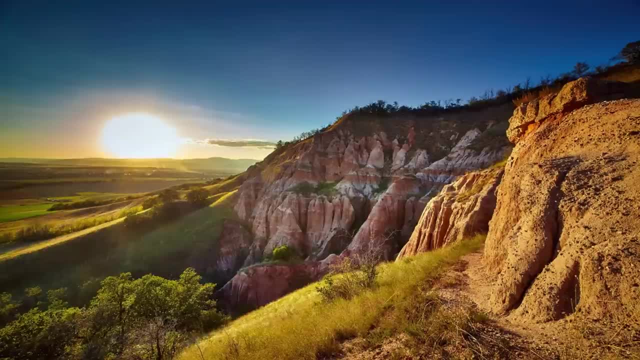 Each day, I awaken with an attitude of gratitude. Each day I awaken with an attitude of gratitude, I let go of all tension that is within me. I let go of all tension that is within me. I am open to a deep calmness inside me. I am open to a deep calmness inside me. 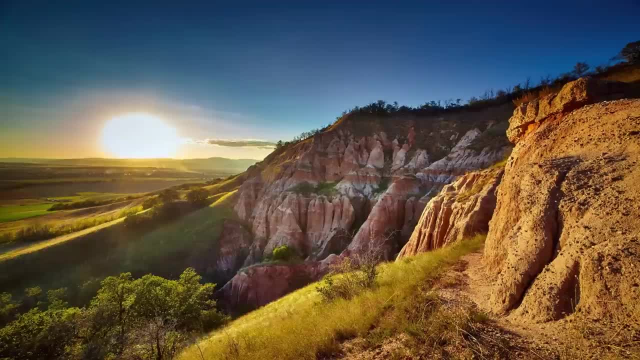 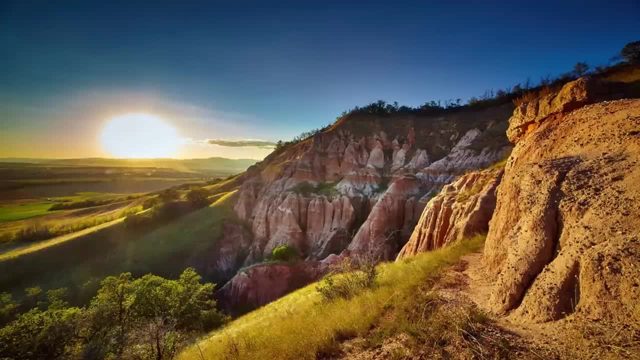 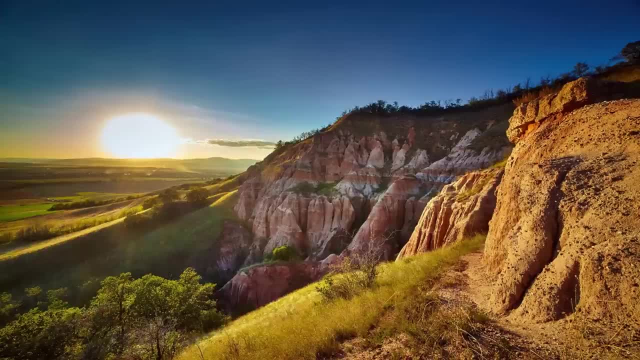 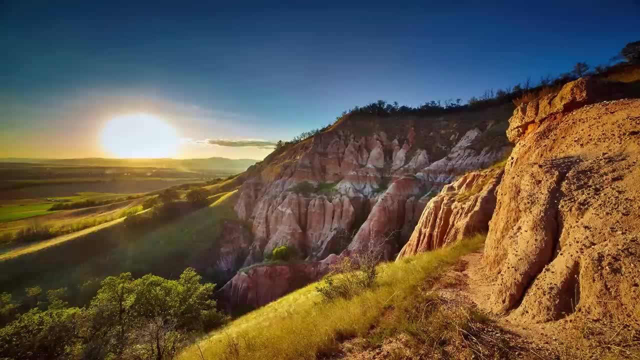 calmness inside me. I am open to a deep calmness inside me. I am open to a deep. I release all thoughts that no longer serve me well. I release all thoughts that no longer serve me well. I create my own happiness in my life. I create my own happiness in my life. 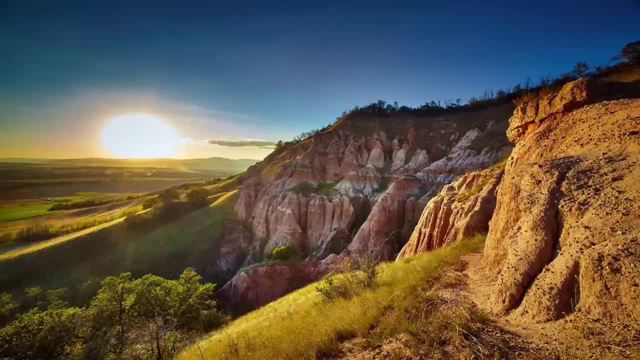 I allow my thoughts to drift to a. I allow my thoughts to drift to a. I allow my thoughts to drift to a positive and peaceful place. positive and peaceful place. positive and peaceful place. I allow my thoughts to drift to a. I allow my thoughts to drift to a. 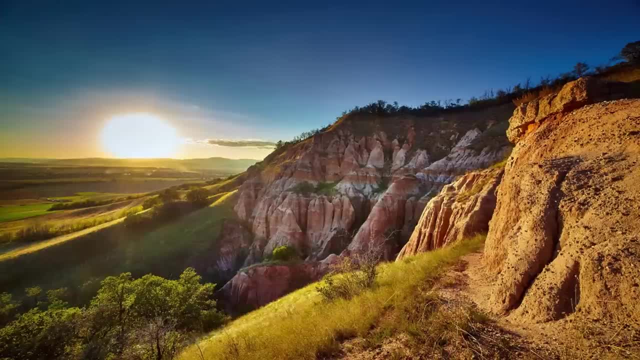 I'm making every effort to forgive myself. I'm making every effort to forgive myself, myself and others. I am always in harmony with the universe. I am always in harmony with the universe. With each breath, I relax my muscles in my body and release tension. 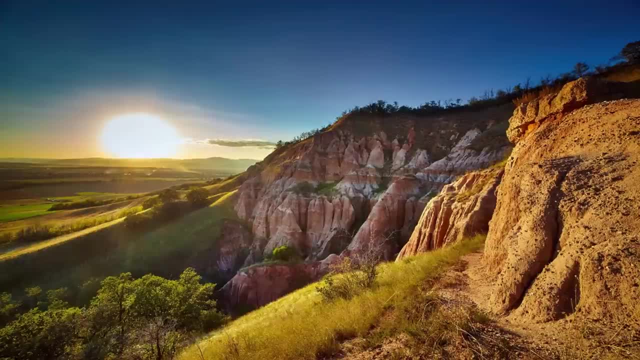 With each breath, I relax my muscles in my body and release tension. With each breath, I relax my muscles in my body and release tension. I am filled with the love of universal power within. I am filled with the love of universal power within. 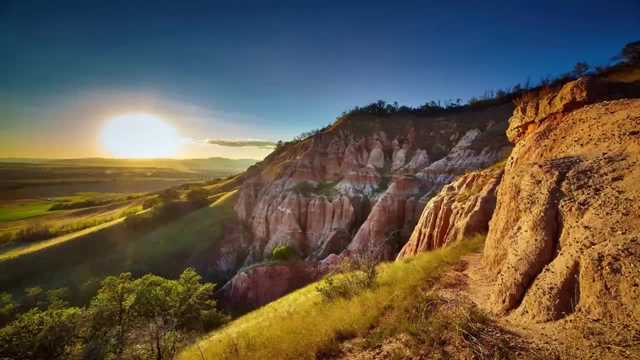 Today, I choose to release all barriers that are holding me back. Today, I choose to release all barriers that are holding me back. Today, I choose to release all barriers that are holding me back. choose to release all barriers that are holding me back. my mind is now free. my mind is now free. 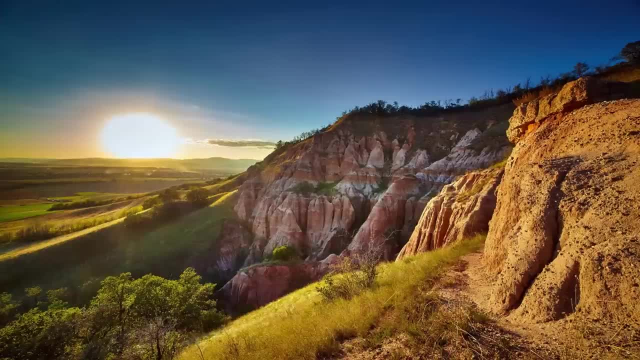 i release any worries of unimportant things. i release any worries of unimportant things with every breath i take. i allow my mind to relax deeply. with every breath i take, i allow my mind to relax deeply. with every breath i take, i allow my mind to relax deeply. 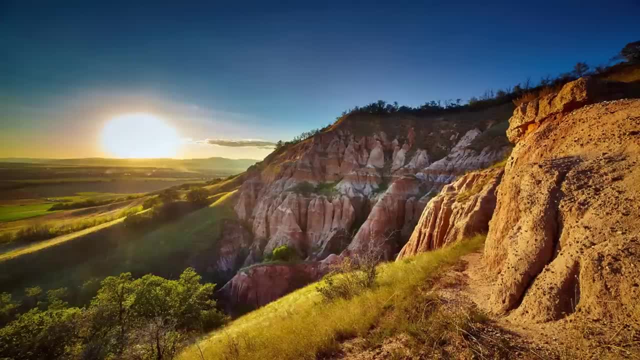 i choose to react in a positive way in all. i choose to react in a positive way in all situations. The things I don't like, I either accept them or can change them. The things I don't like, I either accept them or can change them. 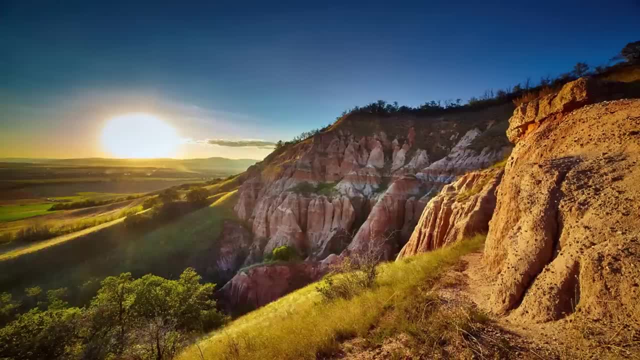 I am what I think, so I choose to think positive thoughts. I am what I think, so I choose to think positive thoughts. On each breath out, I release old negative thought patterns. On each breath out, I release old negative thought patterns. 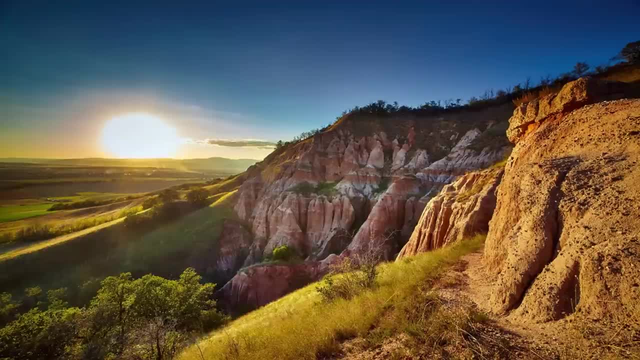 I leave negativity behind. I leave negativity behind. Things are going all right for me today. Things are going all right for me today. All right for me today. Tomorrow is going to be even better. Tomorrow is going to be even better. I create my own space for satisfaction. 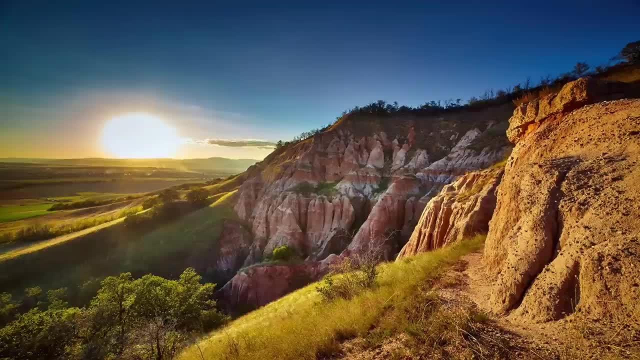 I create my own space for satisfaction. I choose to make happiness my number one goal in life. I choose to make happiness my number one goal in life. Each day, I awaken with an attitude of gratitude. Each day, I awaken with an attitude of gratitude. 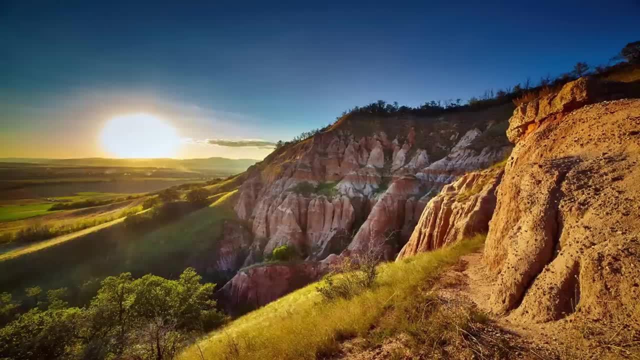 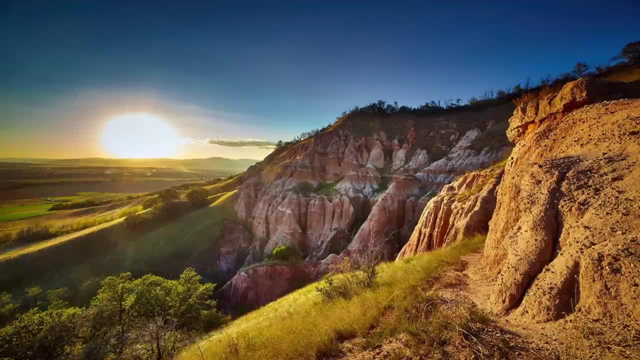 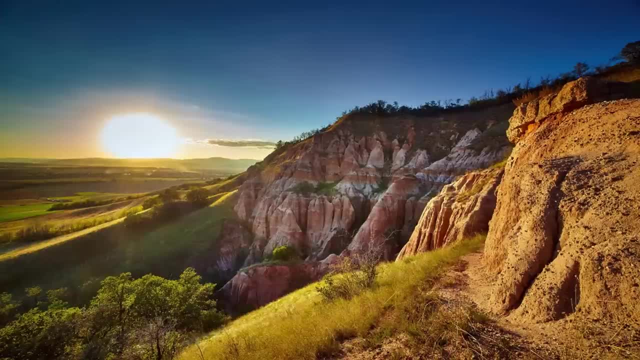 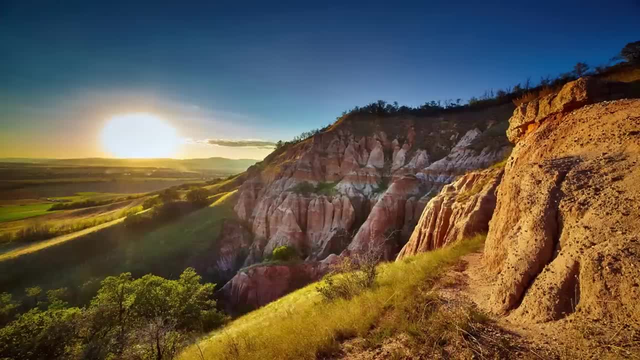 I let go of all tension that is within me. I let go of all tension that is within me. I am open to a deep calmness inside me. I am open to a deep calmness inside me. Right now, I relax my shoulders.